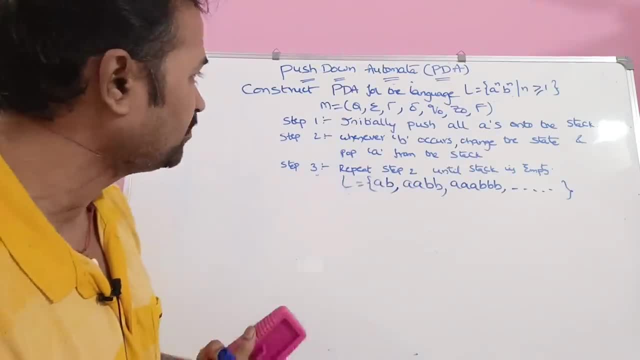 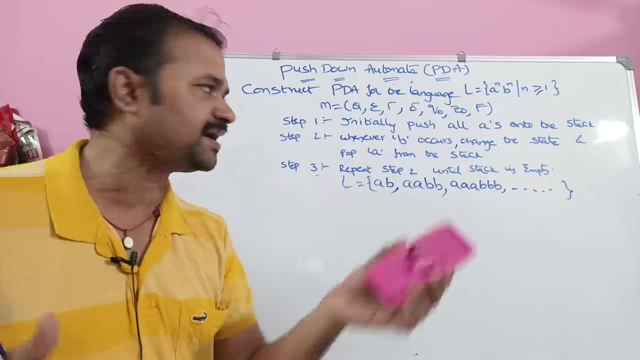 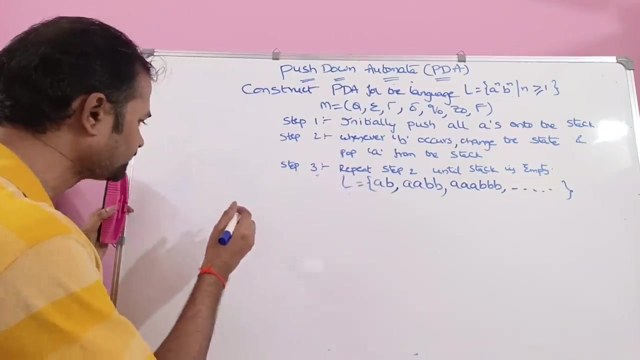 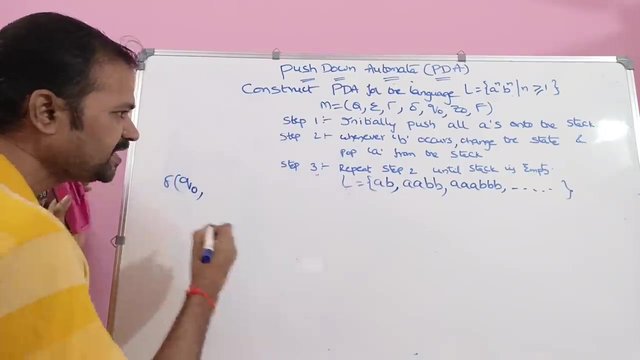 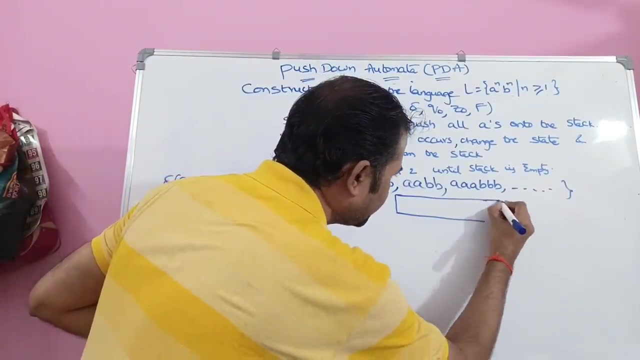 So now let us see the explanation. Now let us calculate the transition function, that is, delta. If we calculate delta, then automatically from the delta we can simply write the remaining 6 doubles also. So let us write the delta. So initially we are at q0 state, So q0 comma Here. first we need to take an input string. Let the input string is: let the input string is 3 bull a, 3 bull b. 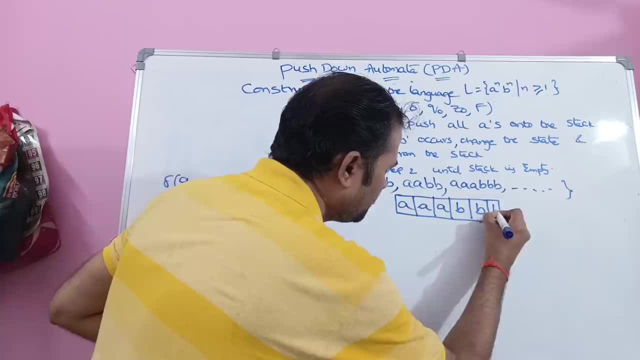 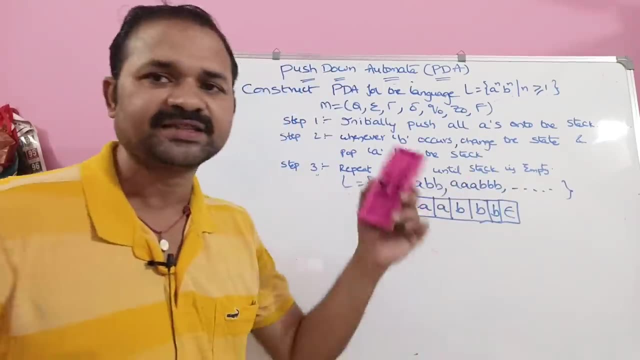 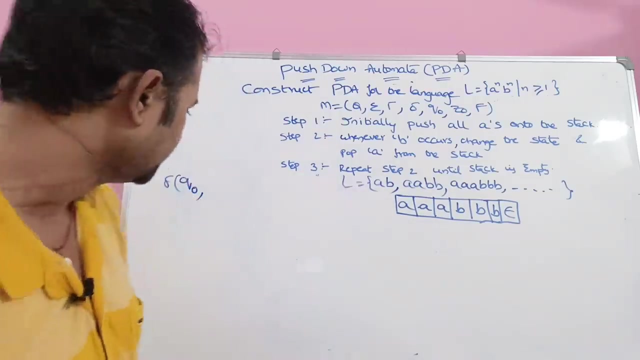 Let, the input string is 3 bull a, 3 bull b, And here the last symbol is epsilon. So if we read epsilon, then it specifies that the complete input string is processable. The complete input string is readable, So q0 comma. what is the first symbol a? 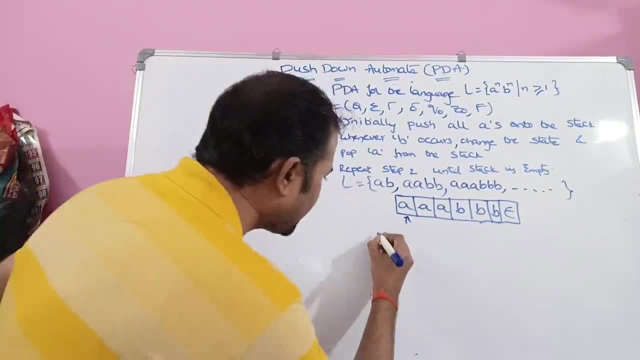 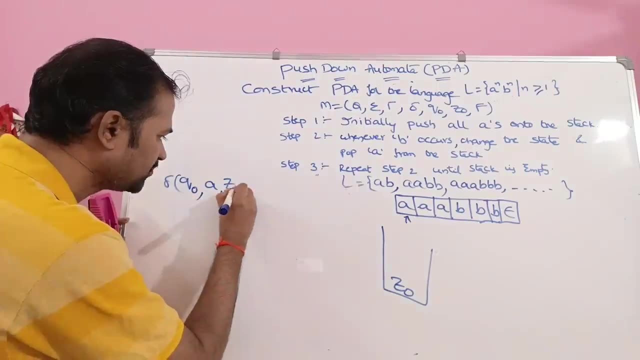 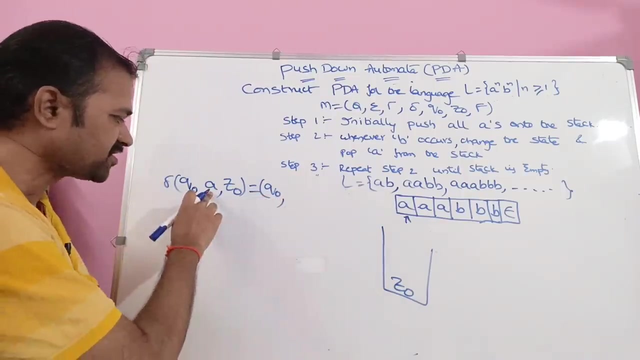 So q0 comma a comma. Initially the stack contains z0.. Initially the stack contains z0.. Here the third argument is z0.. So delta of q0 comma a comma z0 is equal to q0 comma. There is no need to change the state. Why? Because here the input symbol is a. 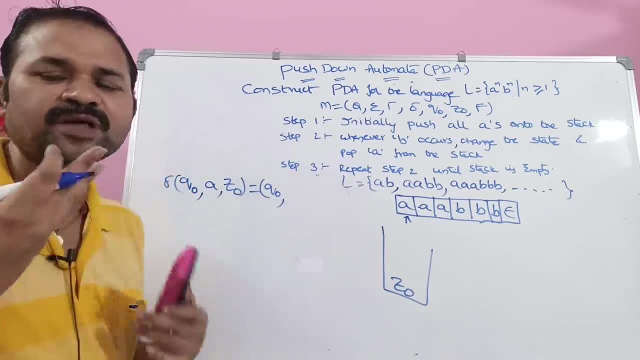 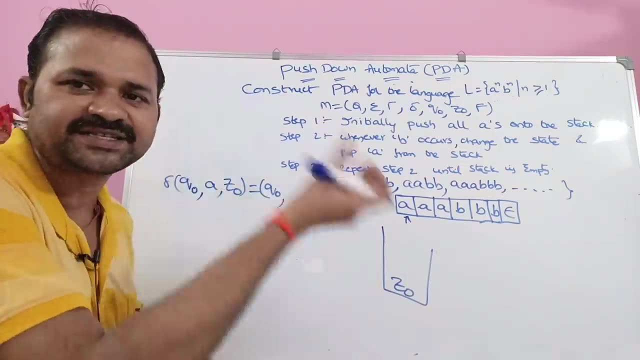 If the symbol is a, then what will happen? We have to do, we have to perform the push operation. While performing the push operation, there is no need to change the state. So here, push means inserting that item out of the stack. Push that item out of the stack. Here, what is the item? a? 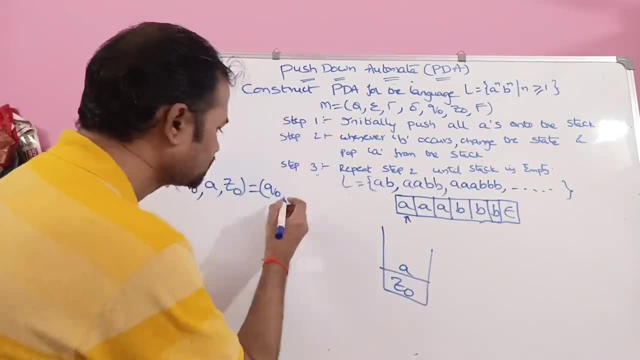 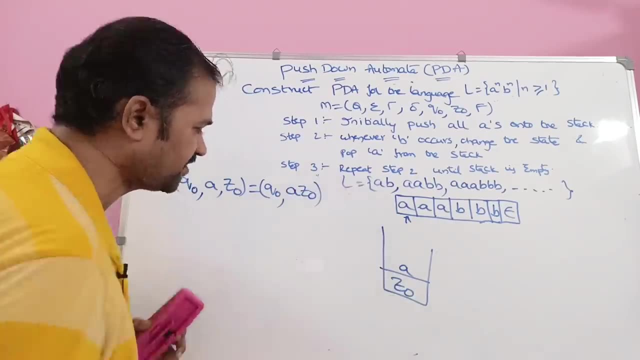 So simply push a out of the stack. So q0 comma. Now the stack contains a and z0.. a and z0.. Stack contains a and z0.. So next one delta of the state is q0, only q0 comma, q0 comma. 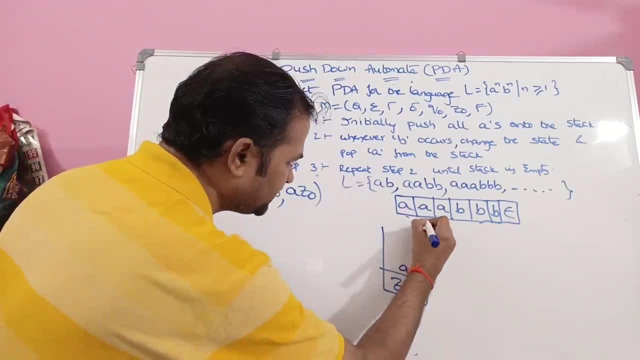 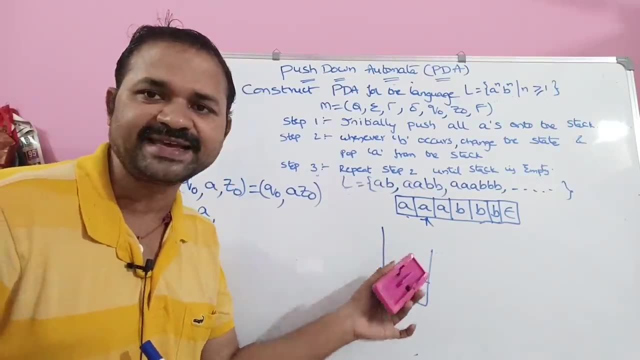 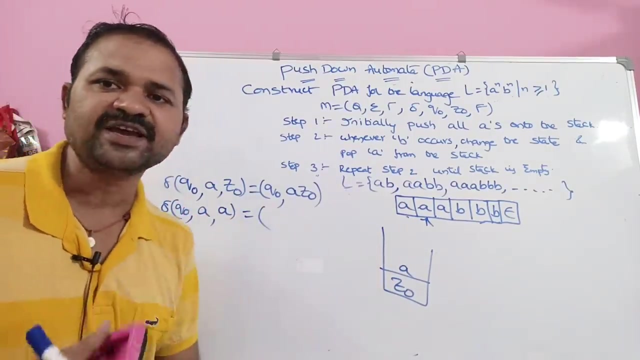 Here this a is readable. The next input symbol is a, only, So a comma. What is the top of the stack? now? The top of the stack is a. So the third argument is: top of the stack is equal to. Here the input symbol is a. If the input symbol is a, then simply we have to push that symbol out of the stack. 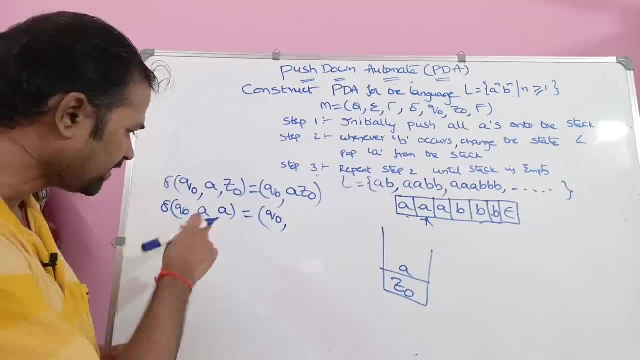 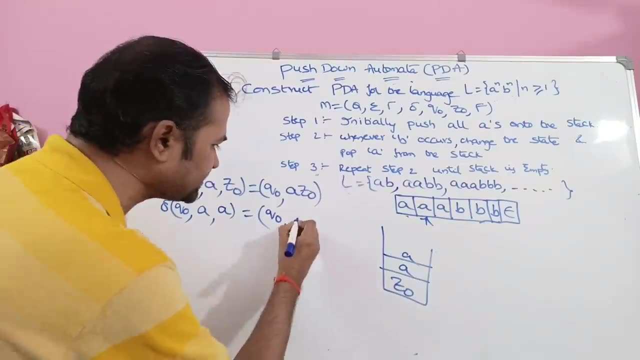 So there is no need to change the state q0 comma. Now we have to push this a out of the stack. So now a will be pushed out of the stack. So now the stack contains a- a z0.. a- a z0.. 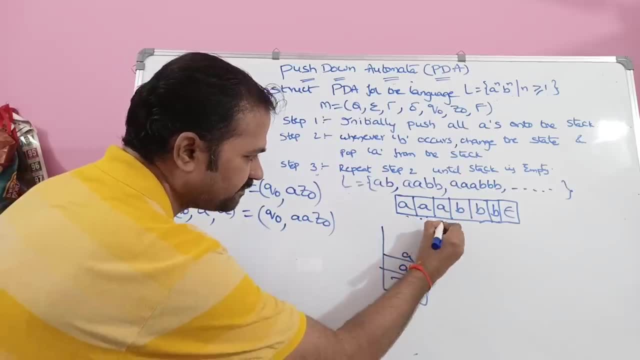 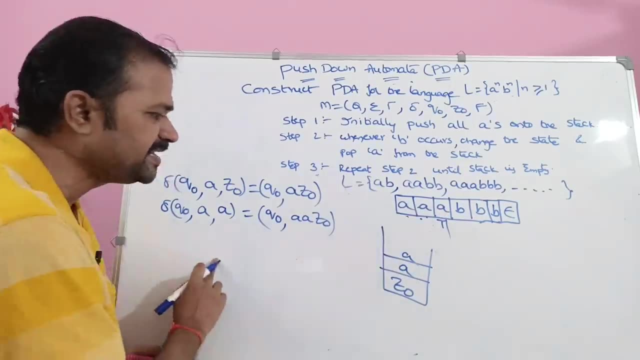 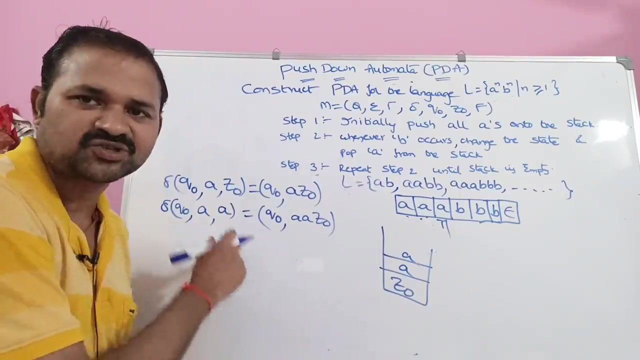 So what is the next input symbol? a. So that is now the extremity- is q0 only, Whereas the input symbol is a and the top of the stack is a q0 comma, a, comma, a. So that is already written. So there is no need to read, there is no need to write the transition one more time. 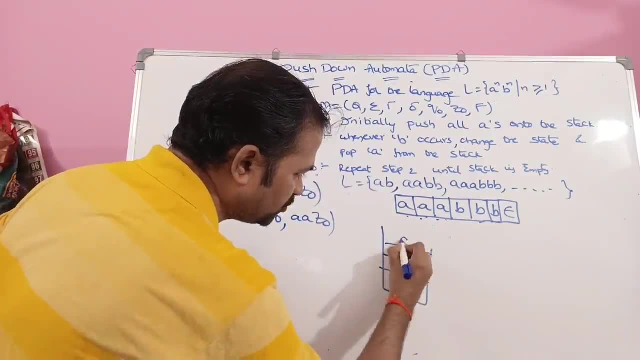 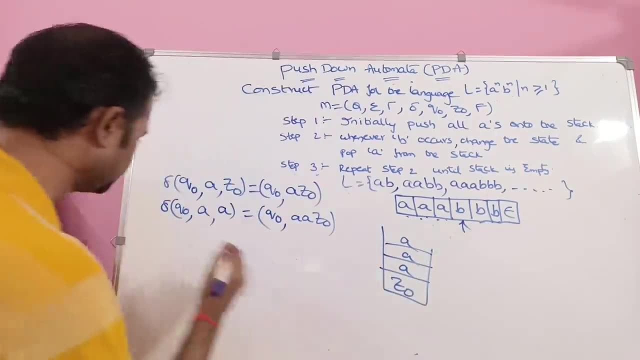 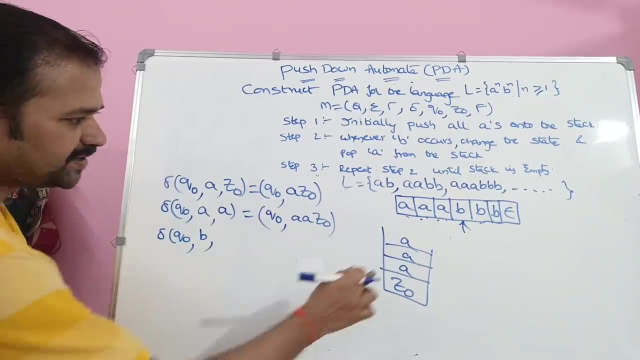 So let us push this. a is out of the stack. So now the stack contains three boolean z0.. So that is what is the next input symbol: b, So delta of q0 comma. So what is the symbol now? b comma, What is the top of the stack? a is equal to. 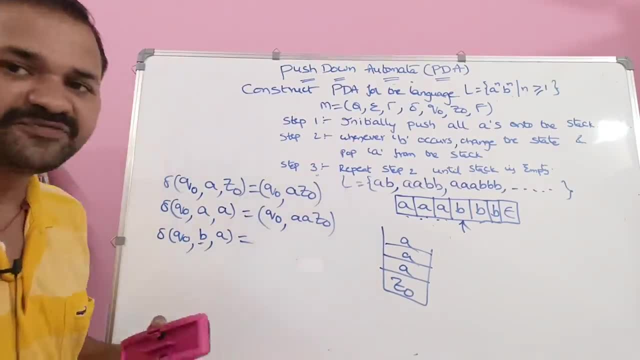 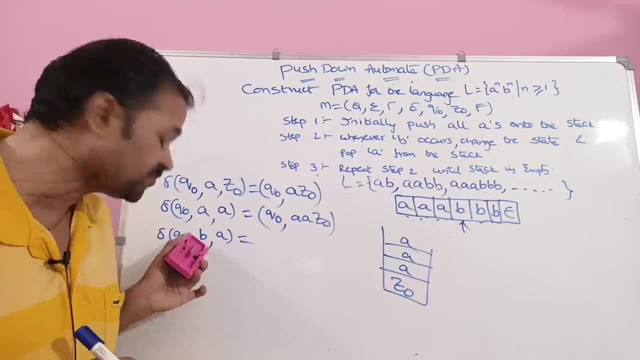 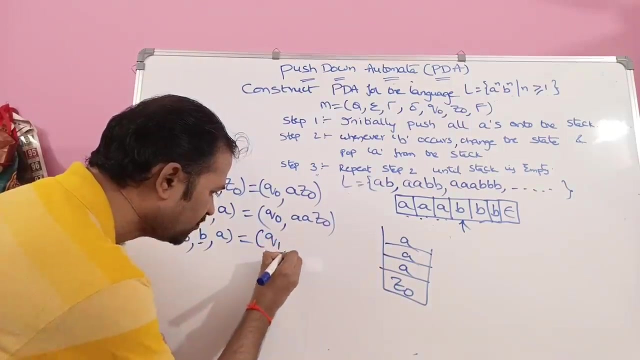 Here the input symbol is b. If the input symbol is b, then what we have to do, We have to perform the pop operation. And for the first pop operation, what we have to do, We have to change the state. So now the state will become q1.. For the first pop operation, we have to change the state. 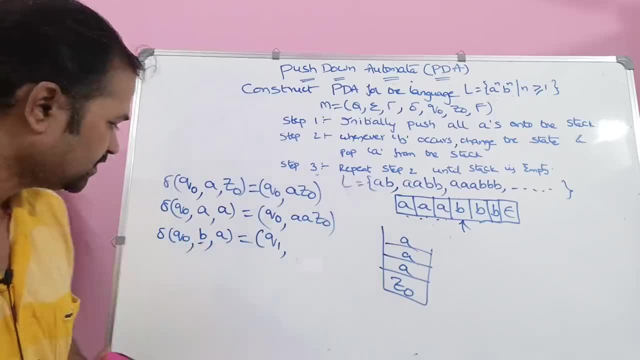 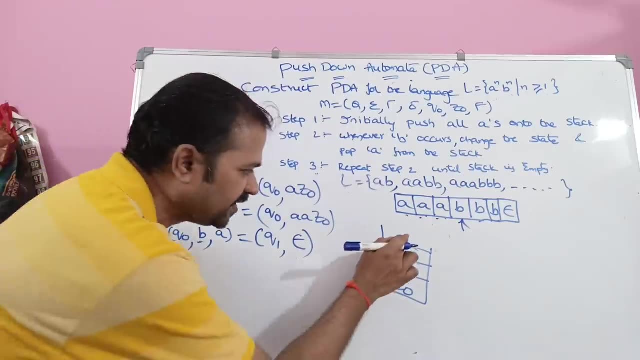 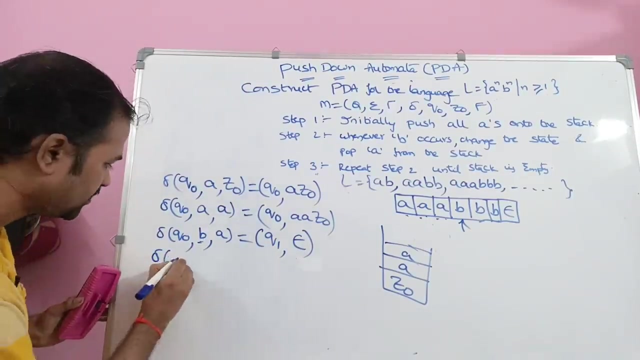 For the next pop there is no need to change the state. So q1 comma. We need to write epsilon. This epsilon specifies that we are performing pop operation. So let us pop this a from the stack. So delta of Now. what is the state now? q1.. q1 comma. 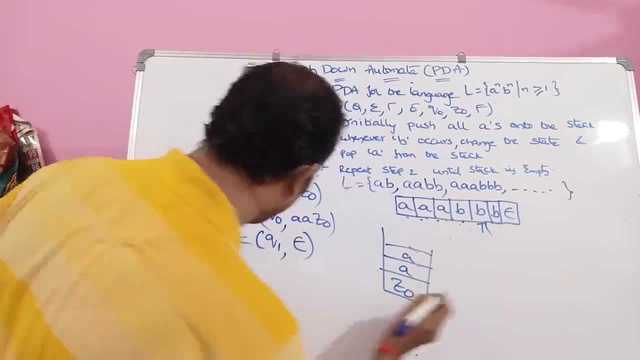 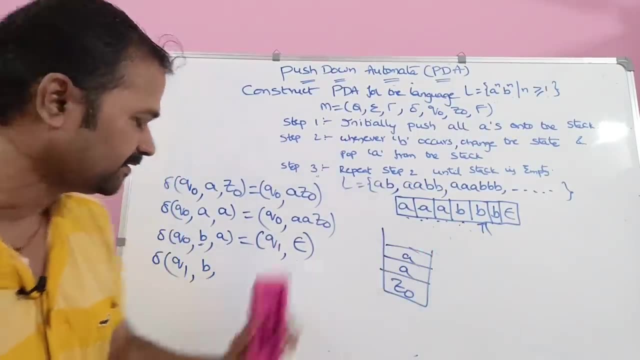 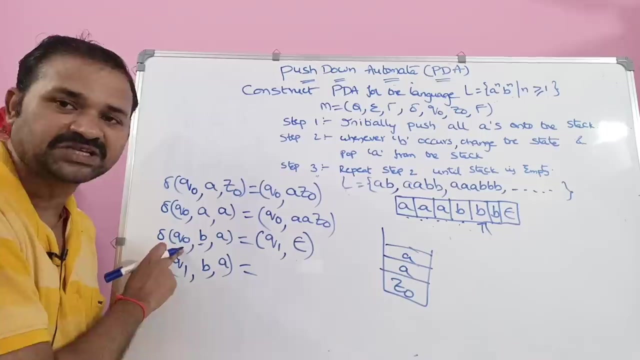 So this b is over. Now let us read this b: Q1 comma. b comma. What is the top of the stack? a? Here there is a difference between this transition and this transition. Here the state is q0.. Whereas here the state is q1.. 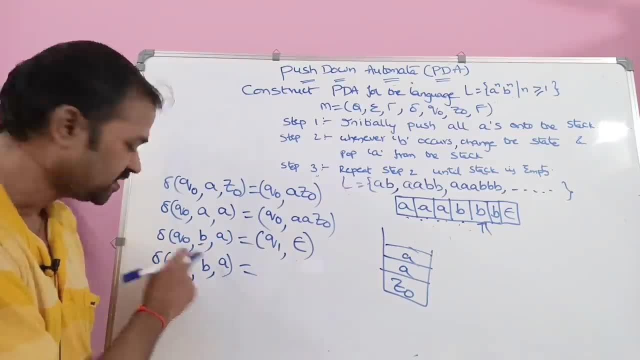 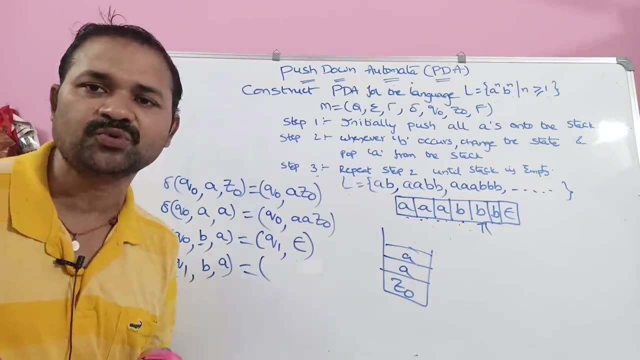 But the input symbols are same and the top of the stack are same, But there is a change in the state. Okay, So here the input symbol is b. What we have to do? We have to perform pop operation Here. this is the second pop operation, So there is no need to change the state. 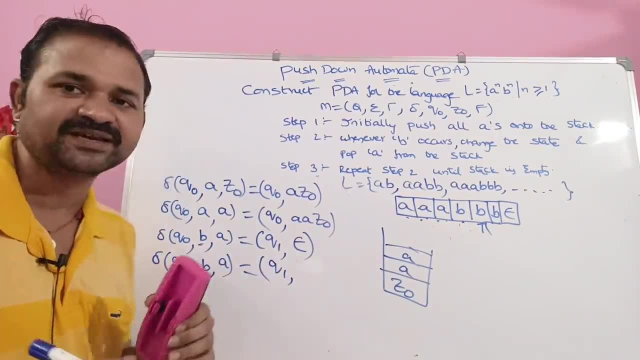 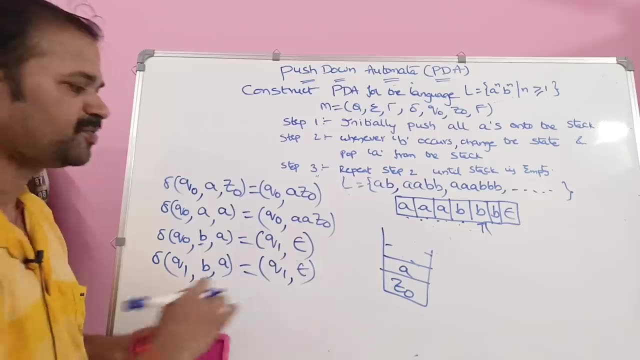 So q1 only. Input symbol is b, So we need to pop the stack. So pop the stack. So now what will happen? This a will be popped from the stack. This a will be popped from the stack. So let us see the next step. The state is q1 only, So q1 comma. 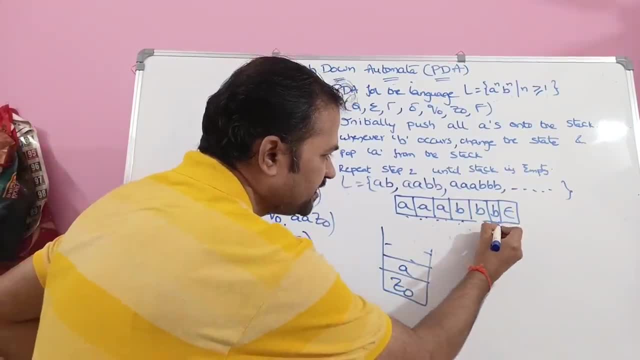 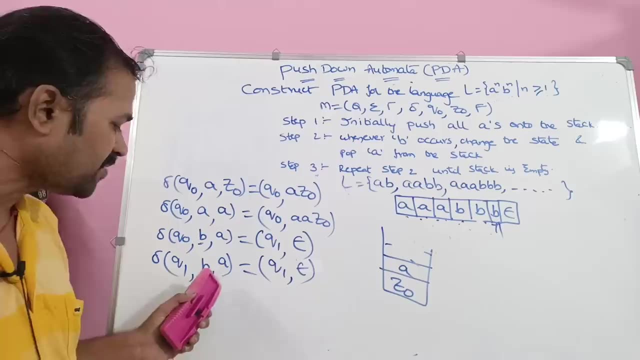 What is the next input symbol? The next input symbol is what b, So q1 comma b comma. What is the top of the stack a, So delta of q1 comma b comma a? That is already written, So there is no need to write that one more time. 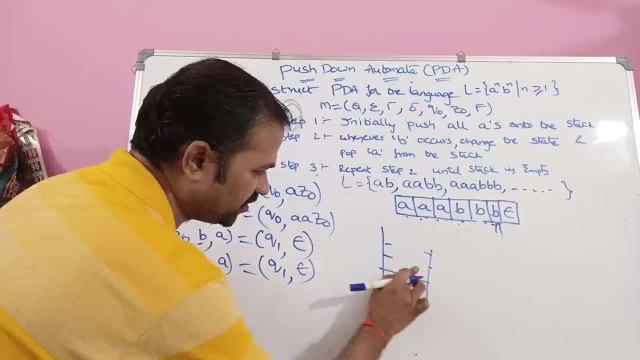 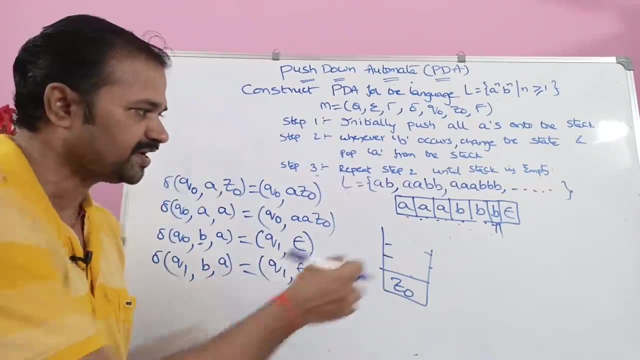 So now what will happen? This a will also get popped, So this is already written. q1 comma b. comma a means what The state is: q1 only, and it will be popped. Okay, So this b is also processed now. So now the input symbol is at what Epsilon? Okay. 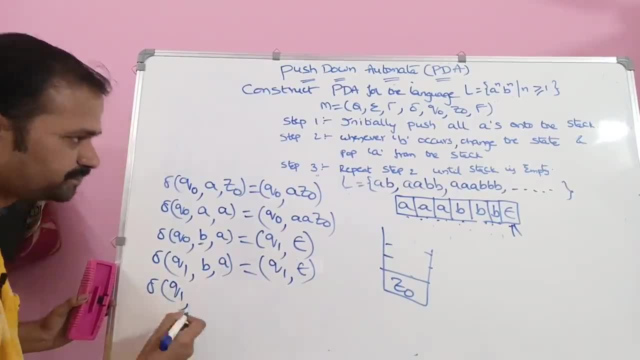 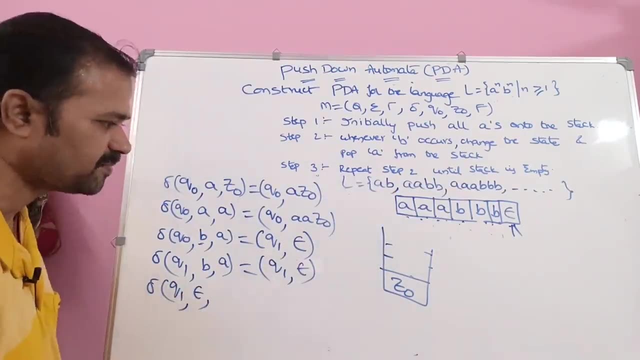 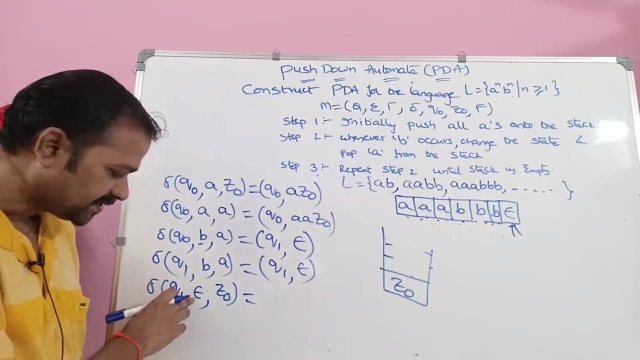 Delta of. What is the state now? q1 comma. What is the input symbol? Input symbol. The input string always ends with epsilon, So q1 comma, epsilon gamma. What is the top of the stack z naught Here? epsilon specifies that this input string is popped. 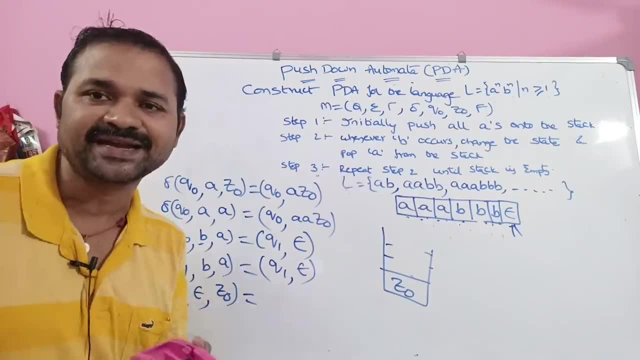 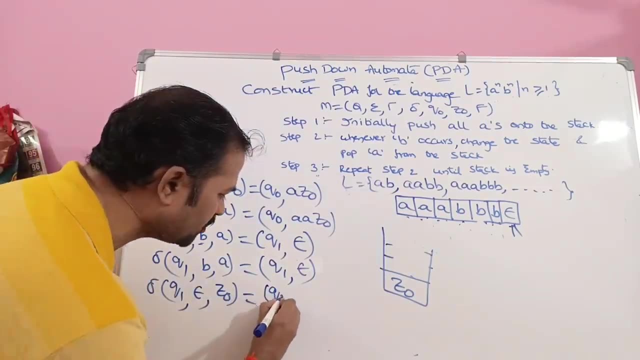 This input string is completely processed, Completely ended. So if the input string is completely processed, then we have to change the state. Let us change the state from q1 to q2.. So q2 comma. Here the stack contains z naught. 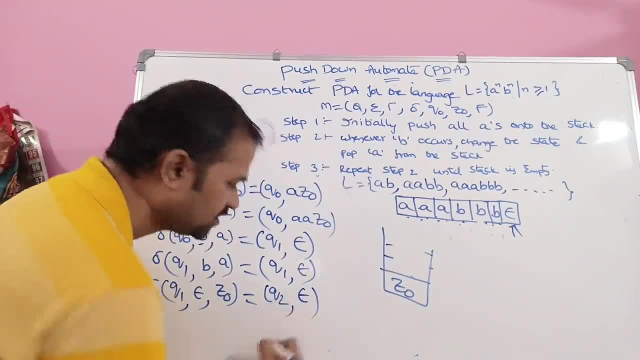 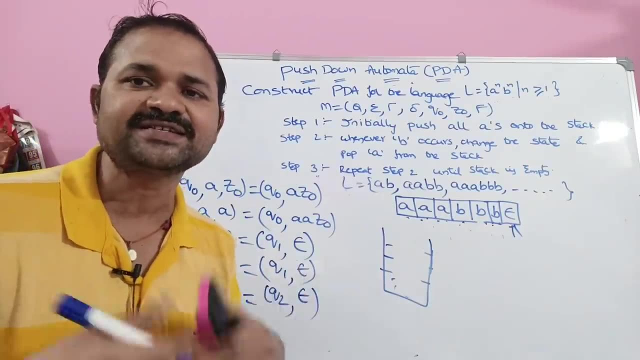 Let us pop the z naught also, So use epsilon. So now what will happen? This z naught will be popped from the stack and the stack is empty. So if the stack is empty, then we can say that the string is accepted by the corresponding string, is accepted by the finite automata. 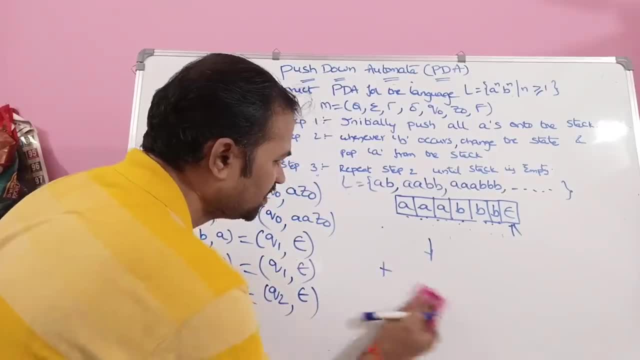 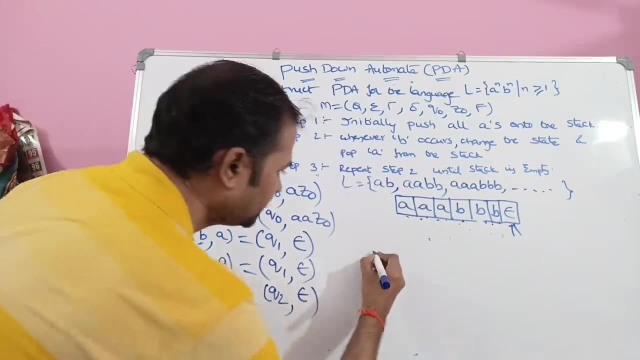 Okay, So these are the transition functions. Now let us draw the diagram, Transition diagram for this one. So, totally, we have how many strings Totally? we have how many strings? Totally, we have three strings. So the first string is q, naught. 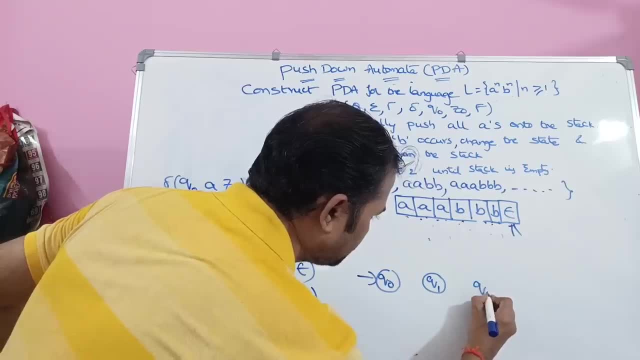 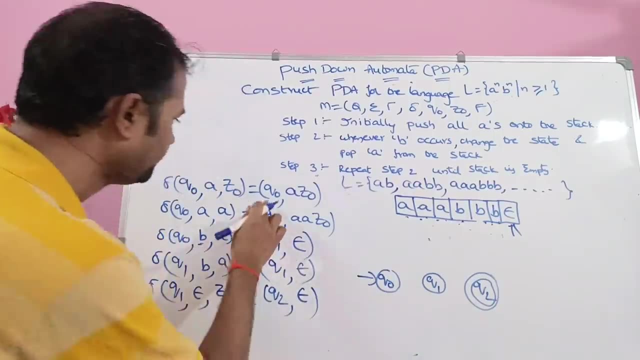 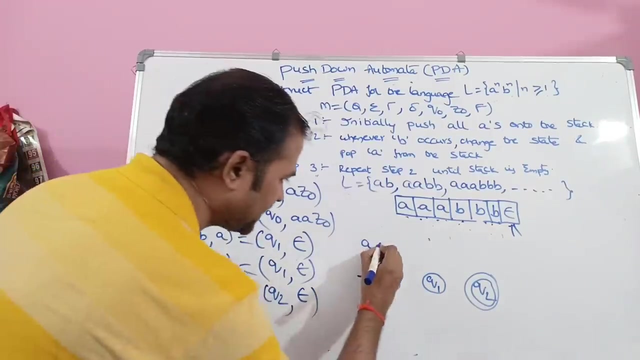 Second string is q1.. Third string is q2.. So this q2 is the final string. So q naught on A will goes to q naught only. So this is self loop. So q naught on A. What is the top most symbol of the stack. 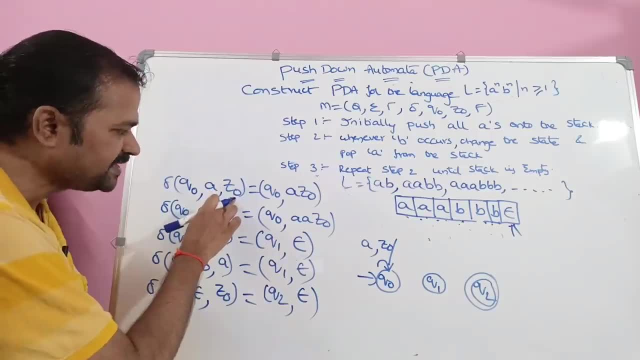 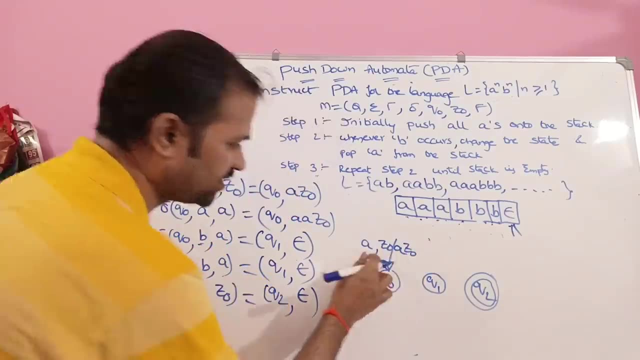 z naught. If the top most symbol is z naught, Then we have to replace this z naught with A z naught. So, slash, we have to write it as A z naught. So it specifies that input symbol is A. 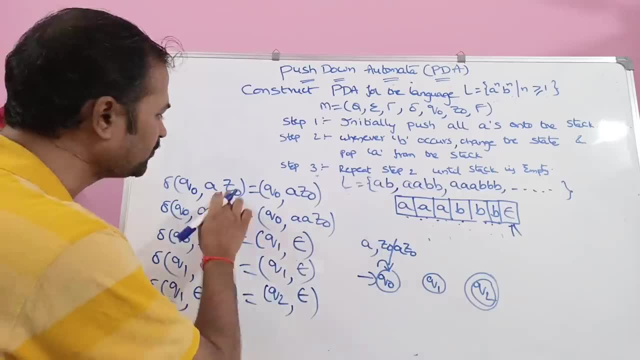 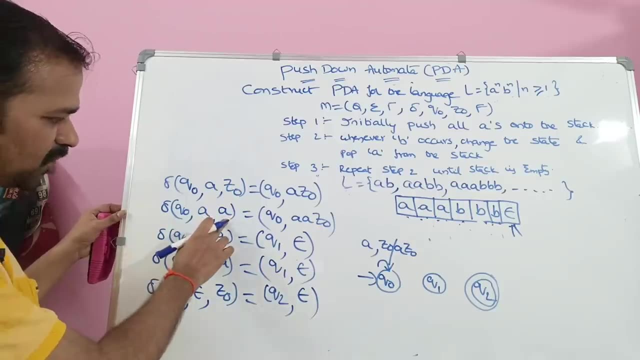 If the top of the stack is z naught, Then we have to replace the z naught with A z naught. Okay, Next one: q naught, A. if the input symbol is A and top of the stack is A, Then it will goes to A naught only. 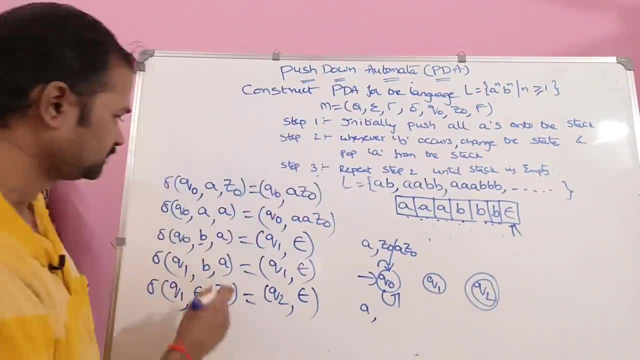 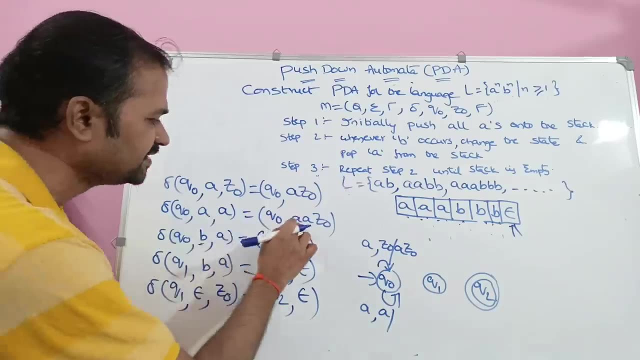 So let us write here A comma. If input symbol is A as well as top of the stack is A, Then we have to replace this A with A A z naught. So let us write here: A A z naught. Okay, So next q naught on B, it will goes to q1. 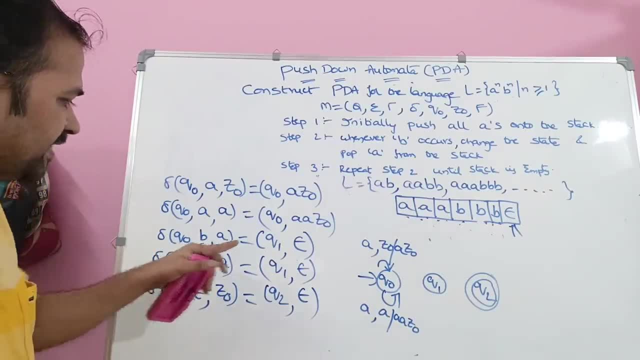 So let us write like this: So q naught on B. If the top of the stack is A, then it is replaced with epsilon. It is replaced with epsilon. Epsilon means simply, we have to perform the pop operation. Next, Next. 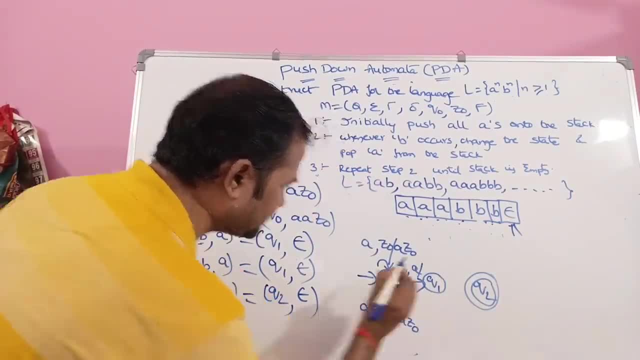 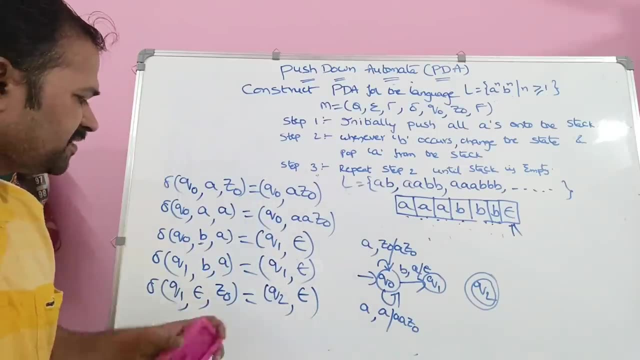 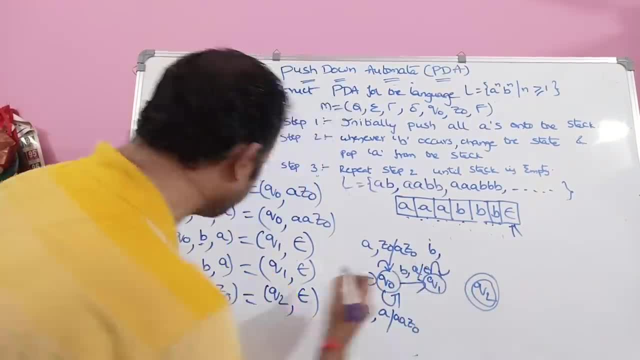 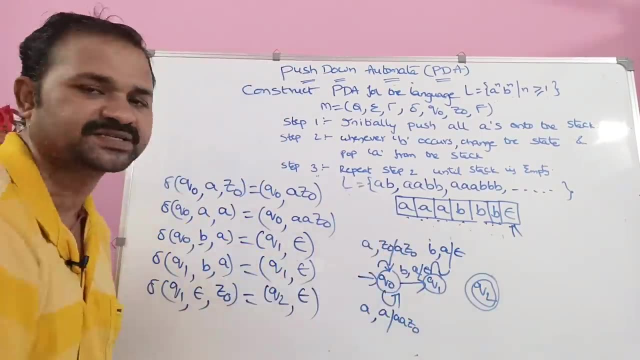 If the input symbol is B, here self loop only, So q1.. If the input symbol is B and top of the stack is A, then simply we have to perform the pop operation. So pop operation means we have to write as epsilon. Okay, 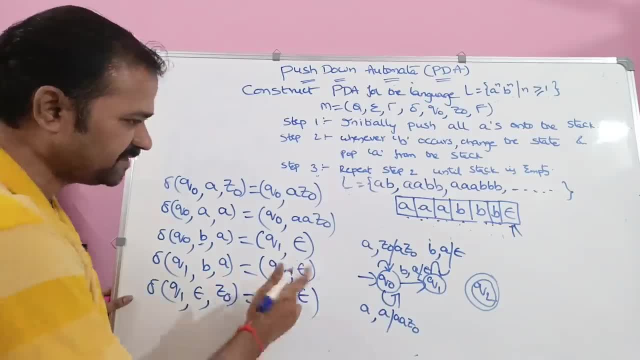 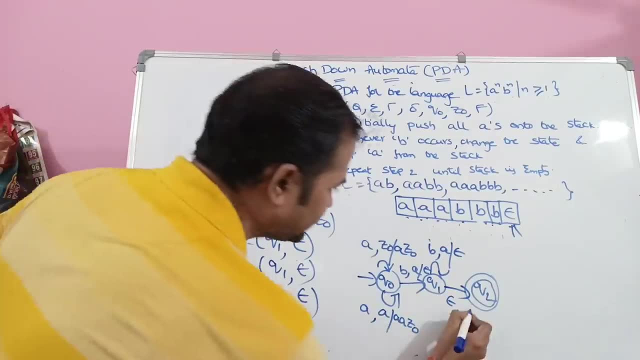 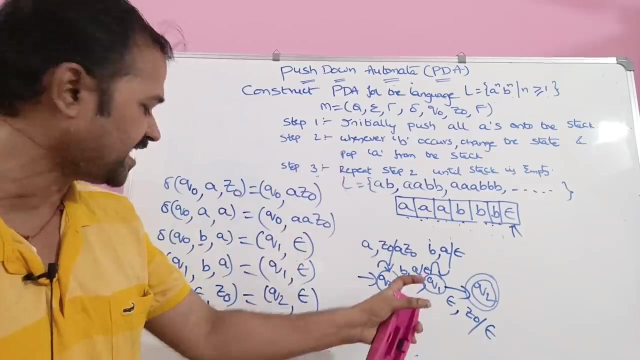 Next to q1.. If the input symbol is epsilon, then we have to go to this state. I am writing here: epsilon. if top of the stack is z naught, then replace with epsilon, then replace with epsilon. so this is the transition diagram. this is the transition diagram. so, according to: 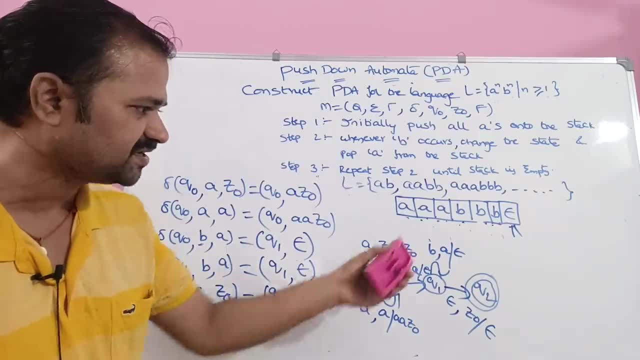 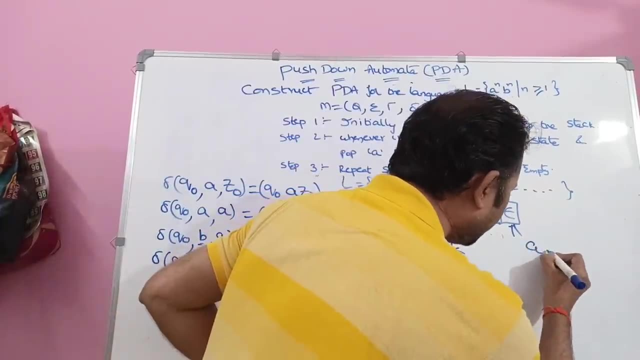 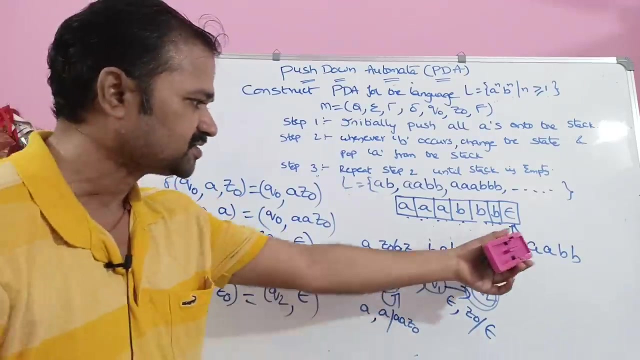 these transitions. okay, first we need to write the transition functions. next we have to wrote down the transition diagram. after that, let us check. let us take a string, any string we can take. let us take a, a, b, b and check whether the string is correctly processed or not. okay, so what is the? 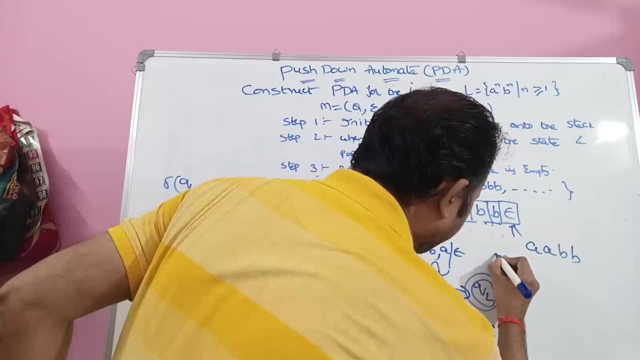 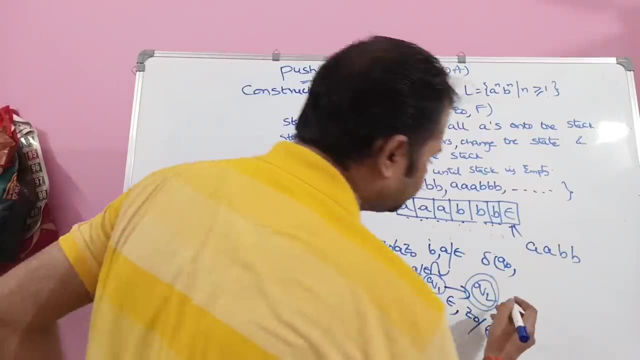 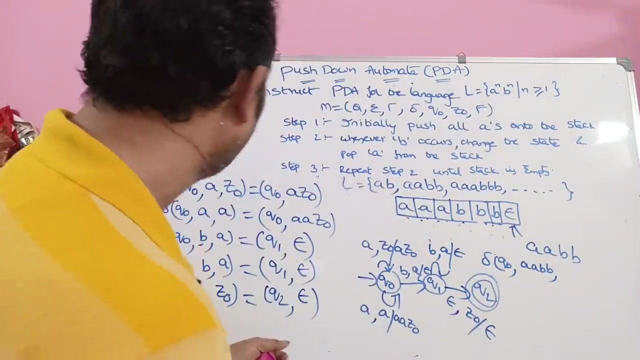 string here: a, a, b, b. so we have to write as delta of q naught power: q, naught power. so what is the string here? a, a, b, b is the string and what is the top of the stack. so let us check whether the string is empty or not. so initially, stack contains: 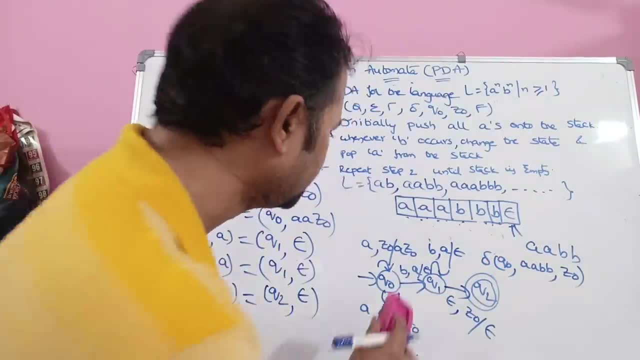 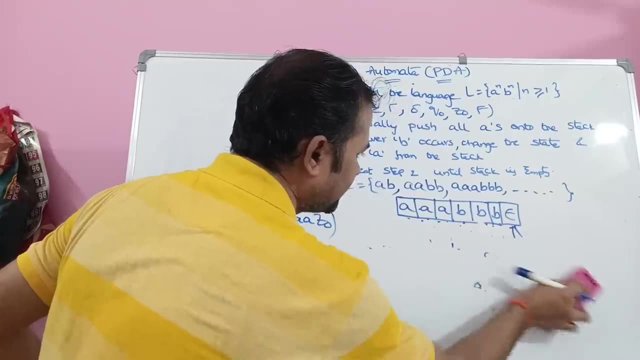 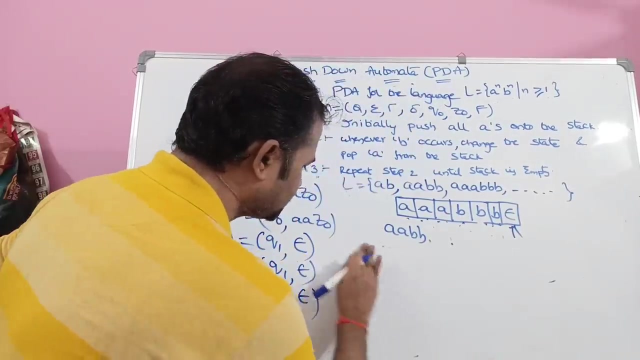 z naught. initially stack contains z naught, so let us write here. let us write here. so if the input string is a a, b, b, a a, b, b, so initially we are at q naught state, and what is the string here? a a, b b. 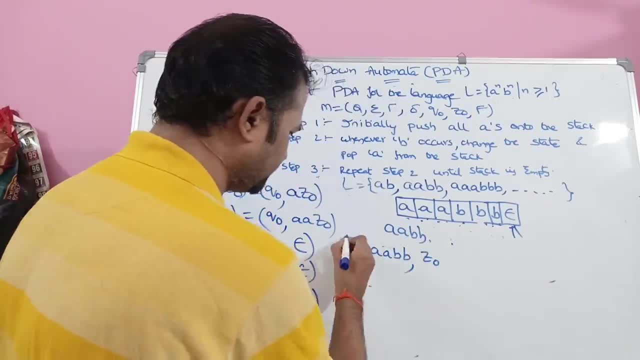 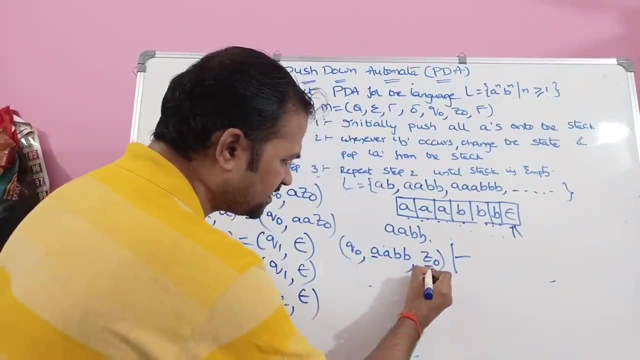 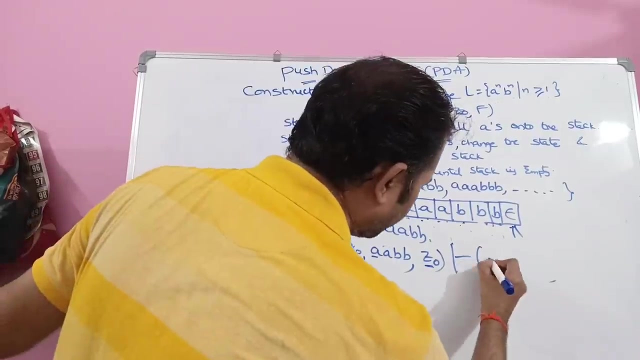 initially stack contains z naught. okay, so input symbol is a top of the stack. is what z naught? input symbol is a top of the stack? is z naught. then we have to move to q naught state. so q naught gamma, q naught gamma. this a is. 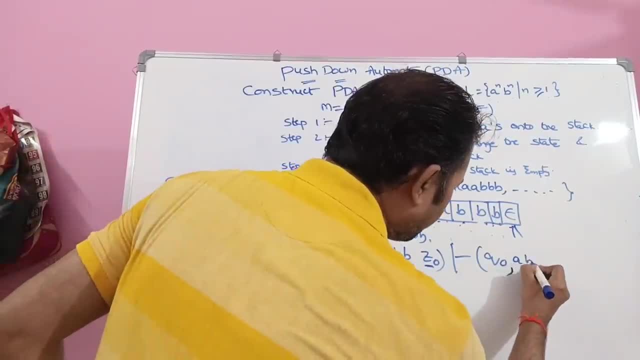 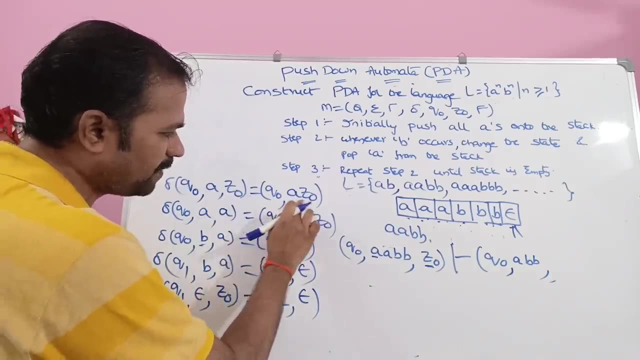 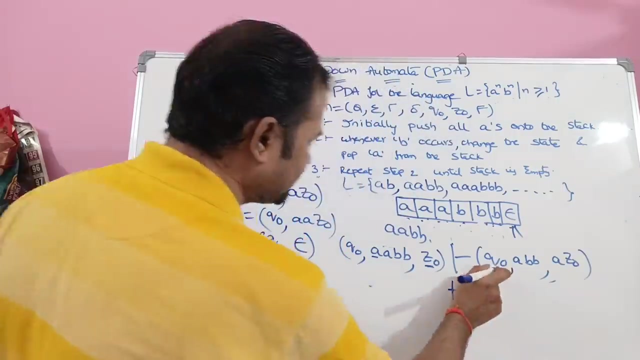 processed. so what is the next input string? a, b, b, gamma. so if the input symbol is a and top of the stack is z naught, then we have to replace with a z naught, a z naught. next, what is the state? q naught is. the state input symbol is a. top of the stack is a, so that is q. 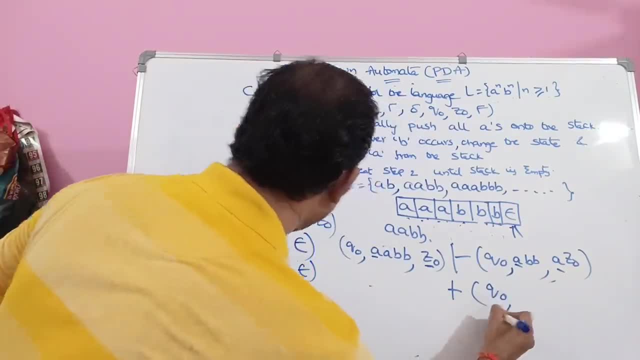 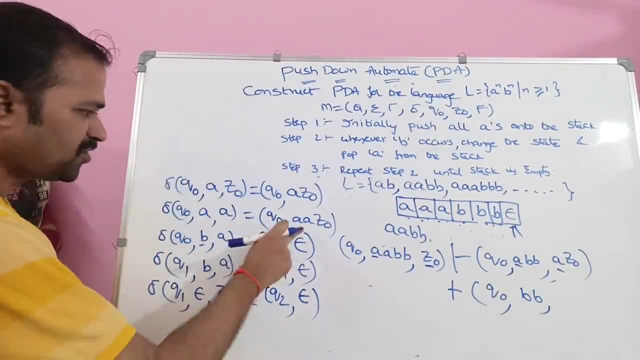 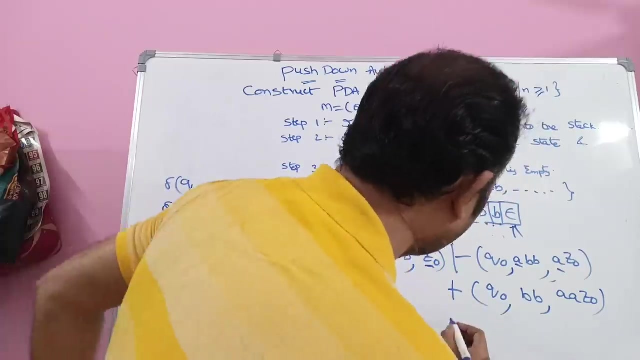 naught a a. then we have to move to the state q naught gamma, q naught, gamma. this a is reading. so the remaining input string is b, b, gamma. so what we have to do we have to push that a out of the stack. so a a, z, naught, a, a, z, naught. next input symbol is what b, top of the. 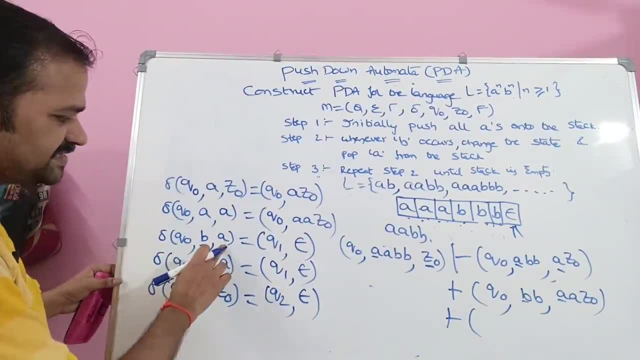 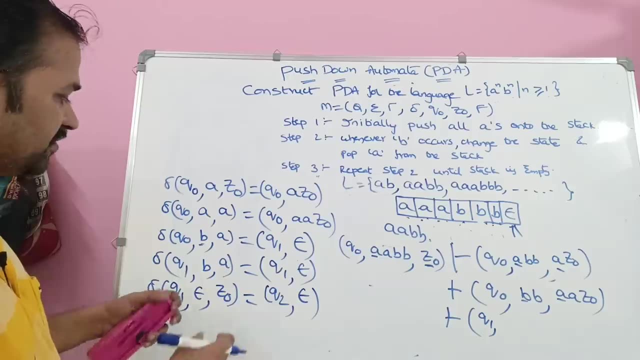 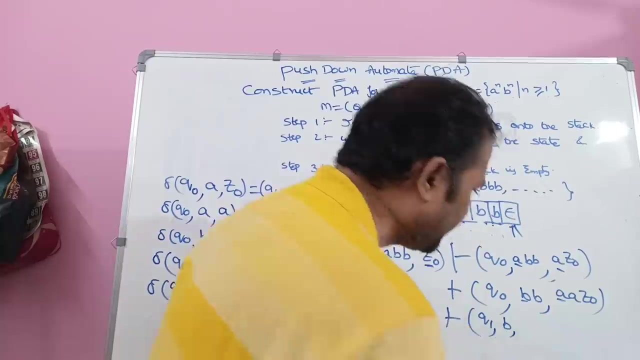 stack is a, input symbol is b, top of the stack is a. then we have to move to the state q 1, so q1 gamma, so q1 gamma. so we need to perform which operation, pop operation. so pop operation means here this b reading is. so next we have b, so we have. 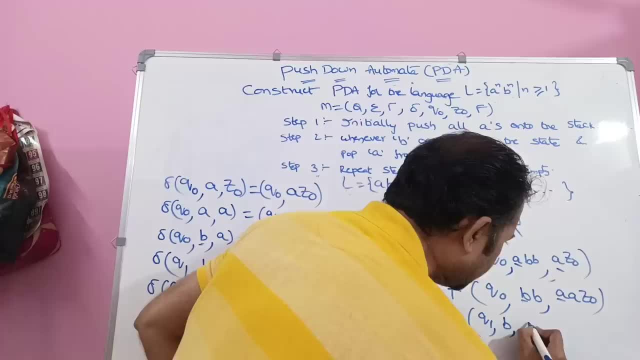 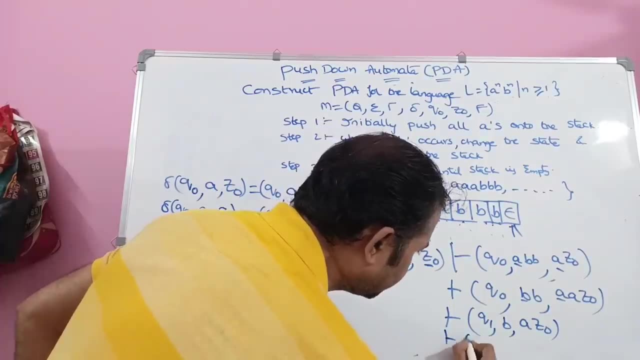 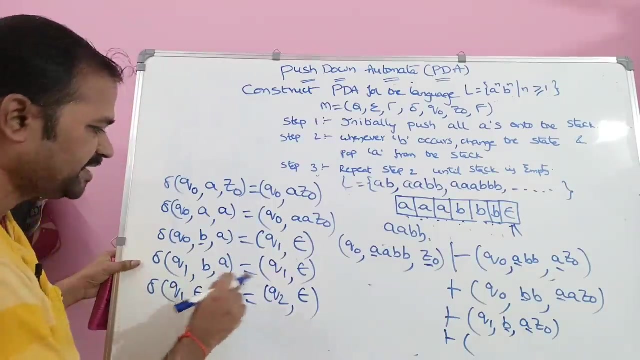 to perform the pop operation. so this a will be from the stack. so now the stack contains a z naught. now the stack contains a z naught. so next Q1, Q1 is the state, input symbol is B and the top of the stack is A. Q1, B A Then 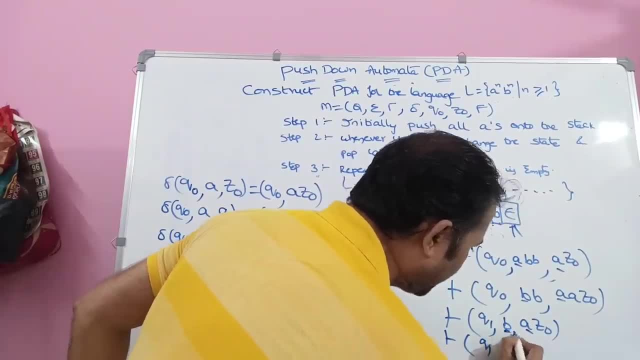 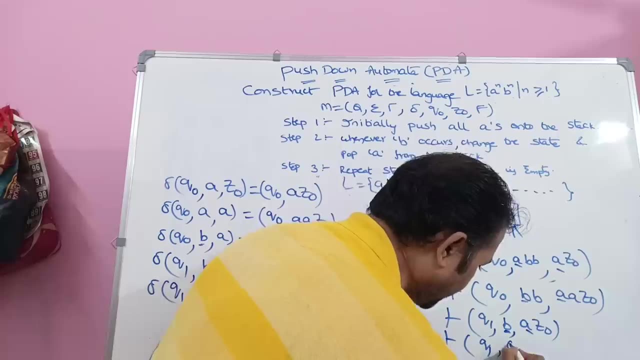 Q1,, Q1,. this B is already over, So we know that the input string ends with semicolon, So here we have to write- I am sorry, epsilon, epsilon, epsilon, comma. Now we have to perform. 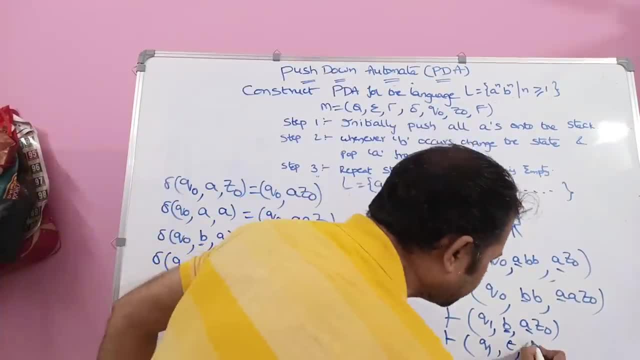 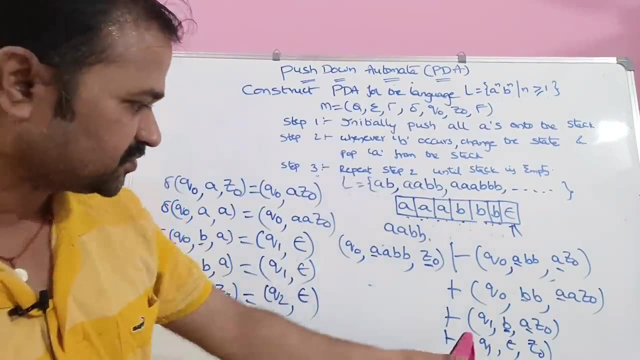 the pop operation Q1, comma- epsilon. Pop operation means this should be this: A will be popped from the stack. So here we have to write: after popping A from the stack we will get Z naught. So Q1, comma- epsilon comma- Z naught. Q1, comma- epsilon comma. 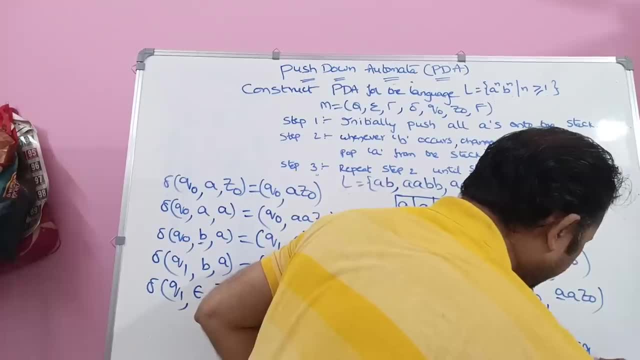 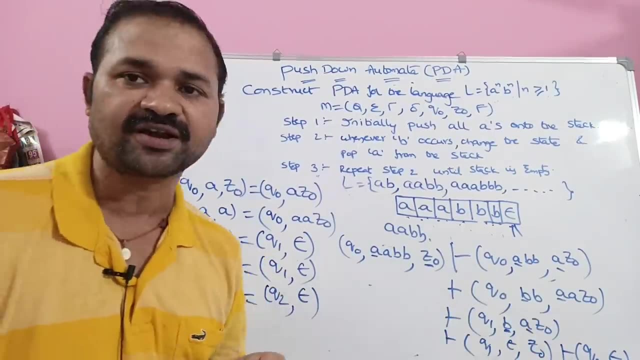 Z naught is nothing but 1.. So for space constraints, I am writing here Q2, comma, epsilon. Here we got Q. what is Q2, final state? as well as we got epsilon. Epsilon specifies that 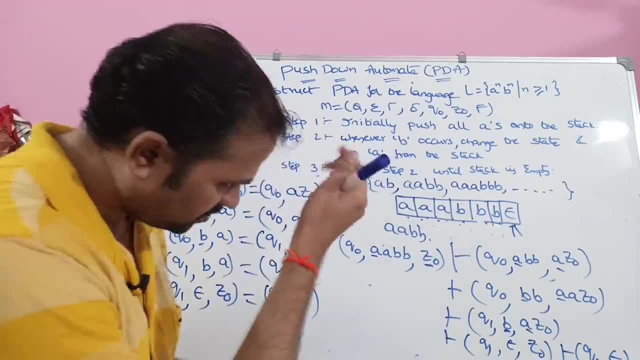 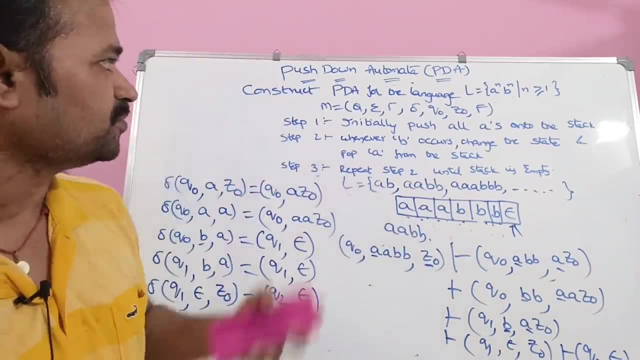 the stack is empty, So we can say that we got the final state as well, as the stack is empty, So this input string is completely empty. This is completely accepted by this push-down automata. Okay, Now let us write the six. 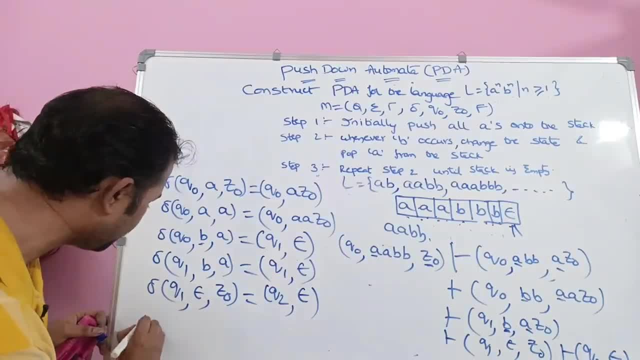 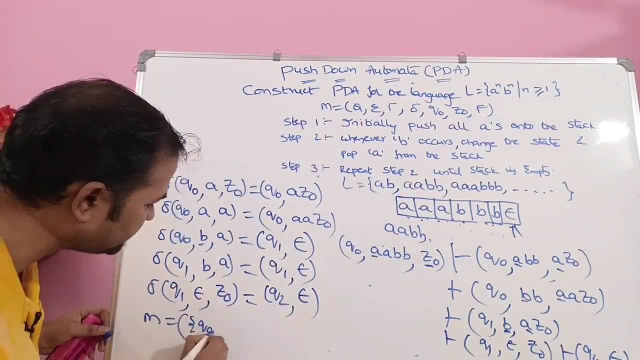 these seven tuples. So first M is equal to Q comma Here totally we have. how many states are there? Q naught Q1, Q2.. So totally, here we have three states are there, So Q. 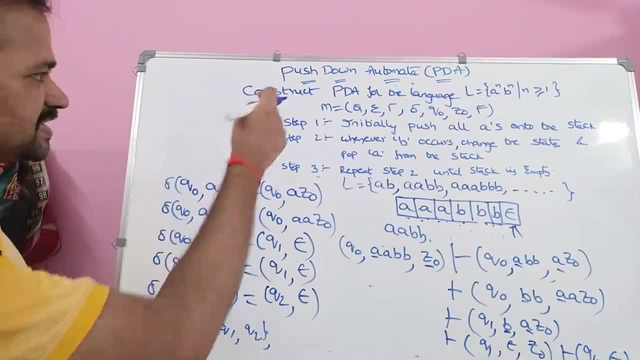 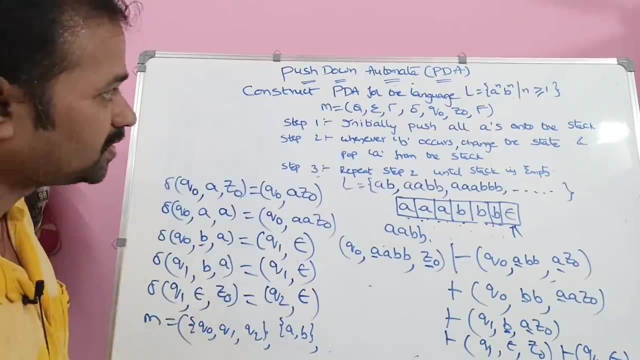 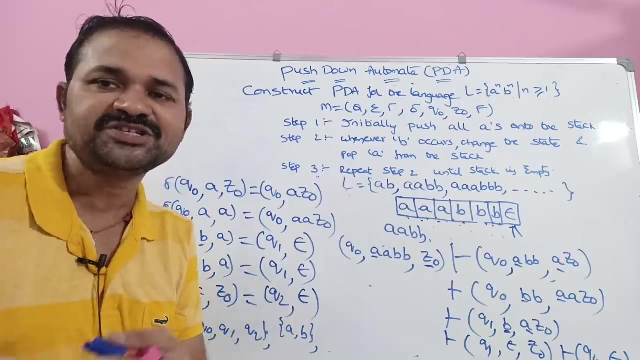 naught, comma Q1, comma Q2.. Next sigma: Sigma means input alphabet. Input alphabet contains two symbols: A and B. Next, tau: Tau means stack alphabet On the stack. what we are doing, we are pushing the symbols. Initially, the stack contains: 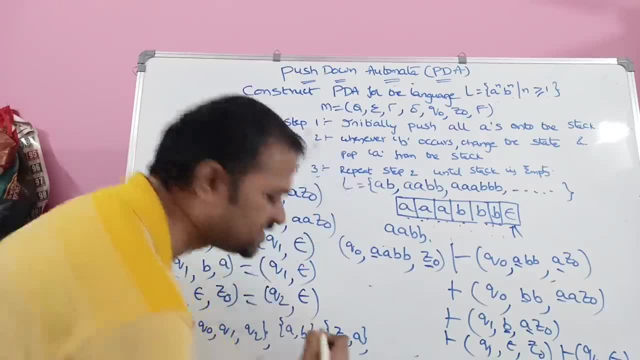 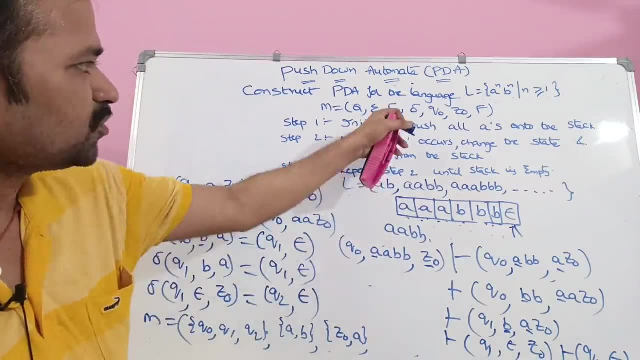 Z naught and we are pushing. A Stack doesn't contains B, So there is no need to write B. If you read B, then simply we are performing the power population. Okay, So tau is over delta. So till now we have calculated delta only. So based on the delta only, we are.